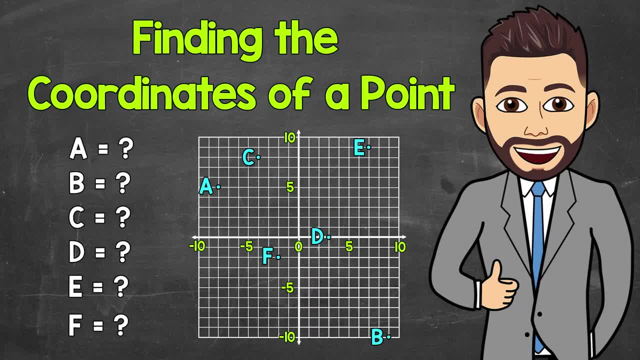 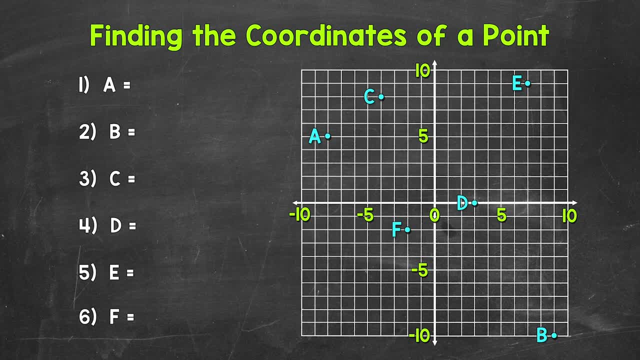 Welcome to Math with Mr J. In this video I'm going to cover how to identify or how to find the coordinates of a point on a coordinate plane. Now, just as a quick review, remember the x-axis is the horizontal axis, so it goes side to side. This is the x-axis right here, And then the y-axis is the vertical axis. 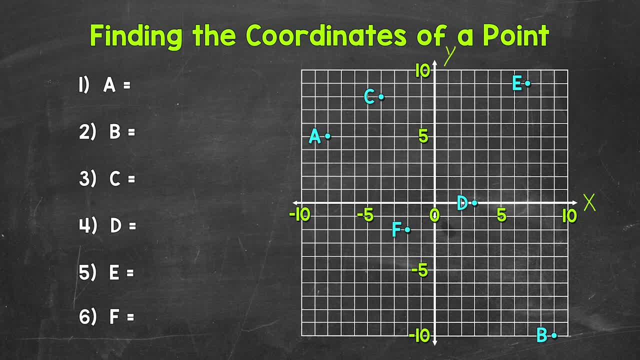 so it goes up and down. This is the y-axis, right here Now remember the x-coordinate always comes first and the y-coordinate always comes second. Let's jump into our examples, starting with number one, where we have point A. So we need to find the coordinates of point A. What's the? 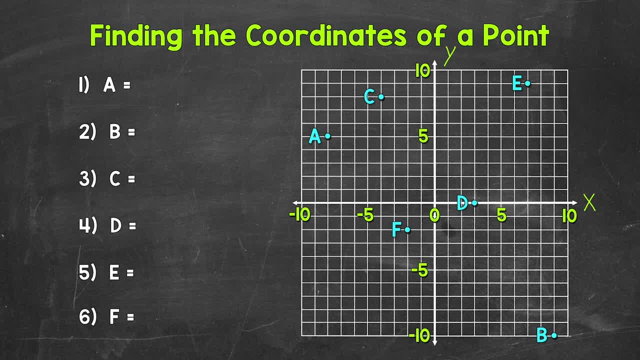 x-coordinate and what's the y-coordinate? So when working with coordinates we always work horizontally. So we need to find the coordinates of point A. So we need to find the coordinates of point A horizontally first. So we need to take a look at the x-axis and where point A is along the 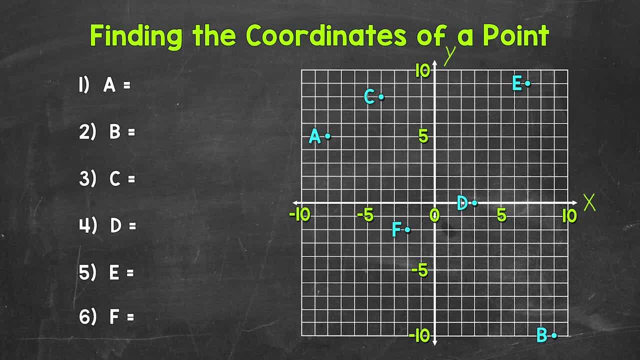 x-axis. So if we take a look at point A, point A is right here along the x-axis and that's negative 8. So that's going to be the x-coordinate. Now we need to find the y-coordinate. So how far up is A? 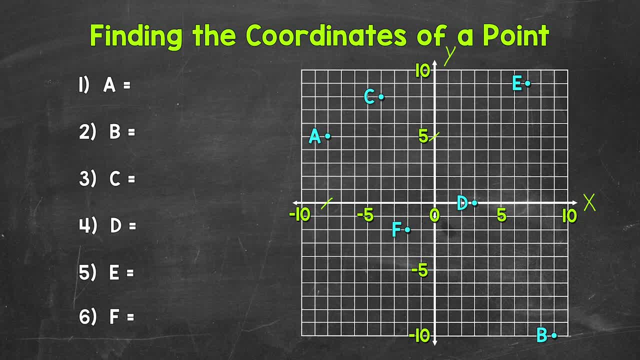 Well, this is 5 on the y-axis, so it's over to negative 8 and then up 5.. So 5 is the y-coordinate, So the coordinates or ordered pair for point A, negative, 8 is the x-coordinate and then 5 is the y-coordinate, So we have x. 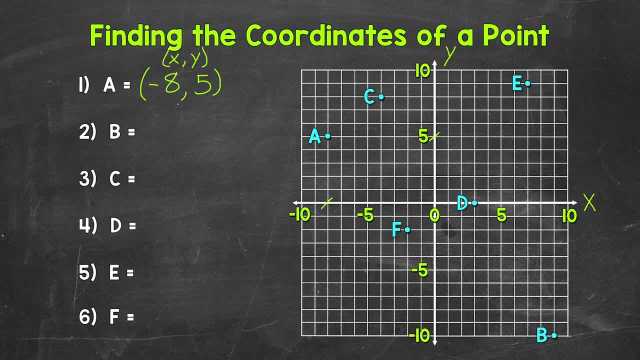 and then y. Let's move on to number two, where we have point B. So let's determine the x-coordinate first. So where along the x-axis is B? Well, right here, which is 9.. So the x-coordinate is 9.. 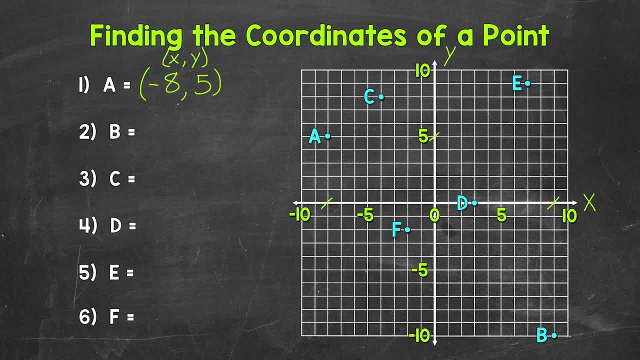 Now we need to figure out the y-coordinate. So how far down from 9 is B? Well, this is negative 10 on the y-axis. So we go over 9 and then down to negative 10.. So negative 10 is the y-coordinate. 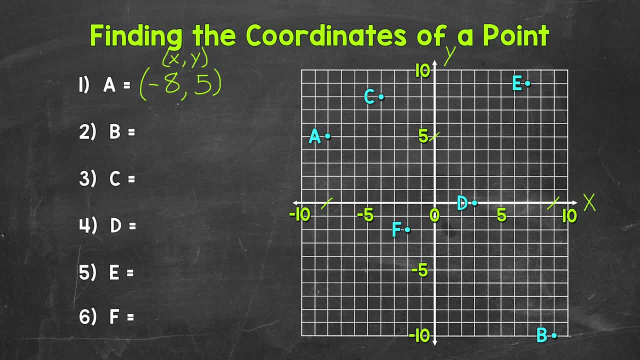 Now we need to figure out the y-coordinate. So how far down from 9 is B? Well, this is negative 10 on the y-axis. So we go over 9 and then down to negative 10.. So negative 10 is the y-coordinate. 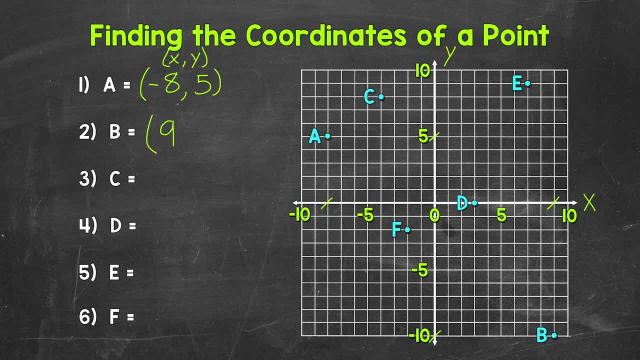 So the coordinates, or ordered pair 9, negative 10.. Let's move on to number 3, where we have point C And we're going to start with the x-coordinate. So where along the x-axis is point C? Well, right here, which is. 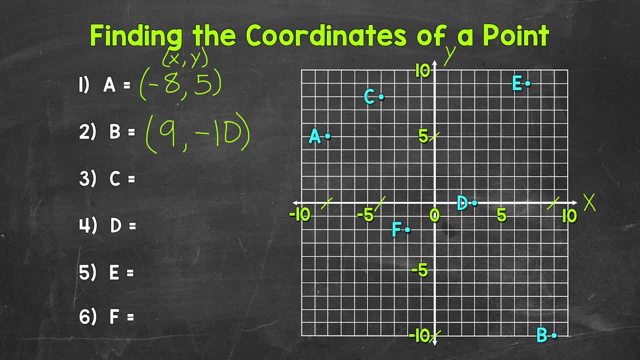 negative 4.. So that's the x-coordinate. As far as the y-coordinate, point C is right here along the y-axis and that is 8.. So the y-coordinate is 9.. So that's the y-coordinate And we're going to 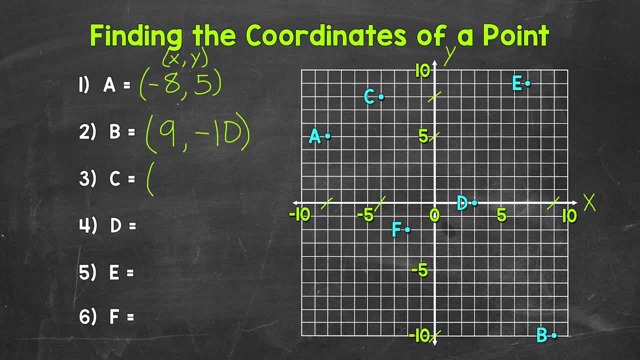 go over to negative 4,, which is the x-coordinate, and then up 8.. So 8 is the y-coordinate. So for point C, we have negative 4, 8.. Let's move on to number 4, where we have point D. So we will start. 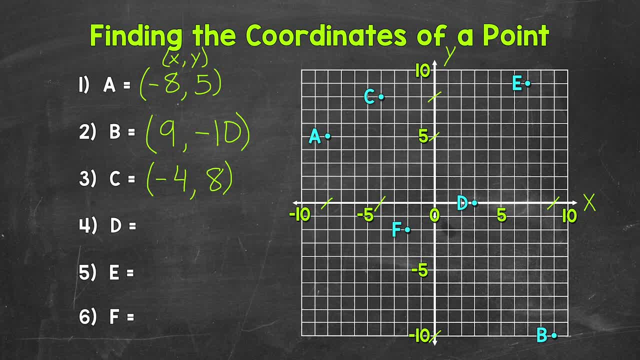 with the x-coordinate. Point D is right here, which is at 3 on the x-axis, And we're going to the x-coordinate is going to be 3.. Now, as far as the y-coordinate, we are at 0 on the y-axis. We did 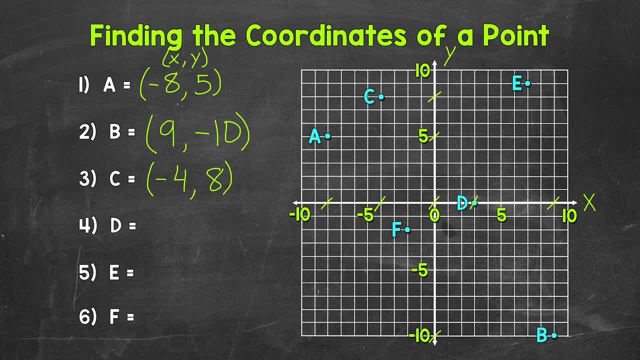 not move up or down vertically, So our y-coordinate is 0.. So for D the x-coordinate is 3, and the y-coordinate is 0.. Let's move on to number 5, where we have point E, And we will start with the x-coordinate. 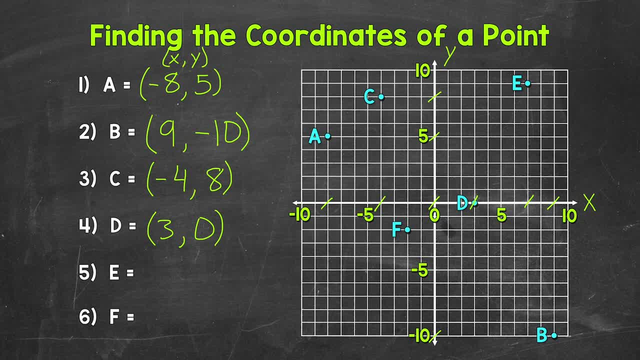 E is right here along the x-axis, So the x-coordinate is 7.. And then as far as the y-coordinate E is right here along the y-axis, So we go over 7 and then up 9 for point E. So 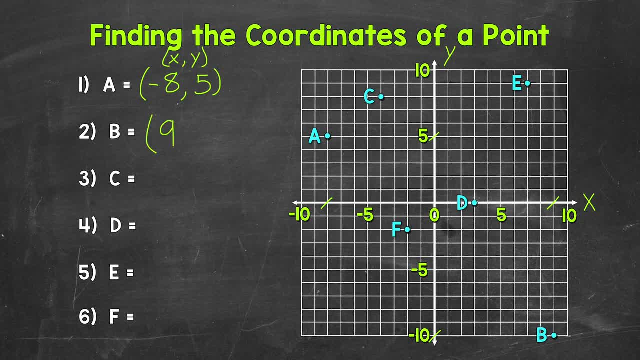 So the coordinates, or ordered pair 9, negative 10.. Let's move on to number 3, where we have point C And we're going to start with the x-coordinate. So where along the x-axis is point C? Well, right here, which is. 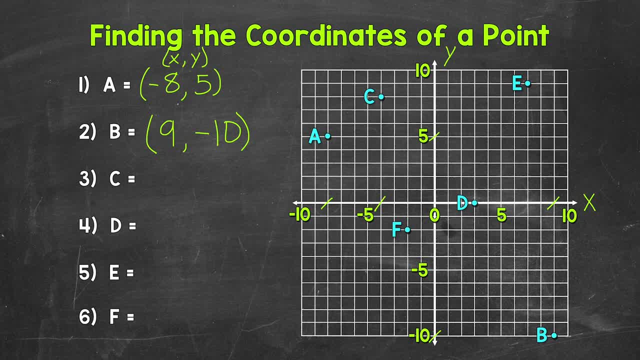 negative 4.. So that's the x-coordinate. As far as the y-coordinate, point C is right here along the y-axis and that is 8.. So the y-coordinate is 9.. So that's the y-coordinate And we're going to 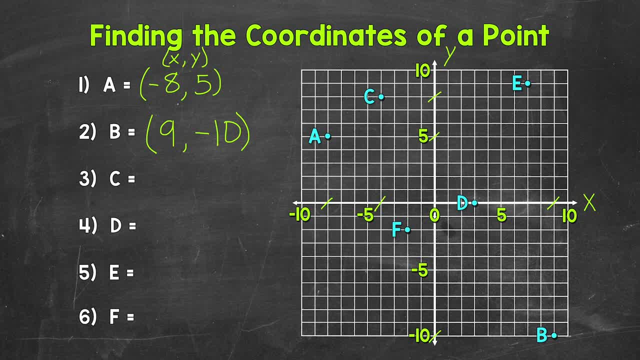 The y-coordinate is 8.. So we go over to negative 4,, which is the x-coordinate, and then up 8.. So 8 is the y-coordinate. So for point C we have negative 4, 8.. Let's move on to number 4, where we have 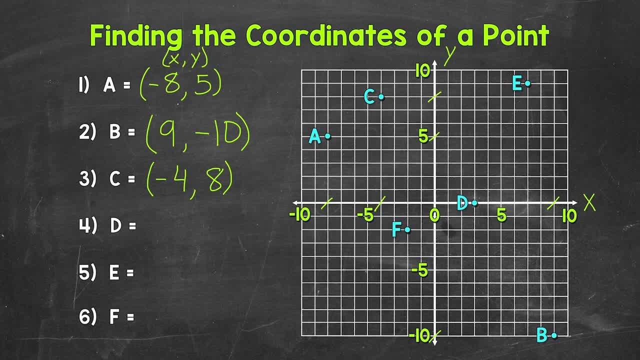 point D. So we will start with the x-coordinate. Point D is right here, which is at 3 on the x-coordinate. So the x-coordinate is going to be 3.. Now, as far as the y-coordinate, we are at 0 on the y-axis. We 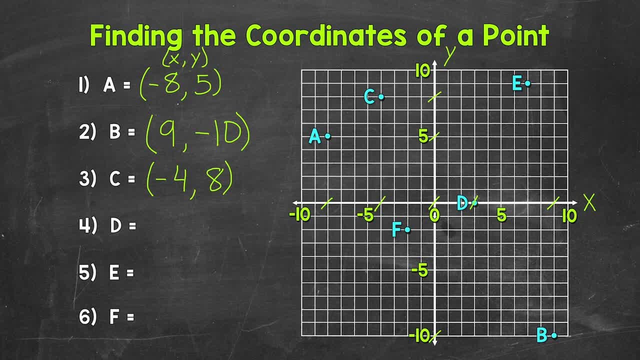 did not move up or down vertically, So our y-coordinate is 0.. So for D, the x-coordinate is 3, and the y-coordinate is 0.. Let's move on to number 5, where we have point E, And we will start. 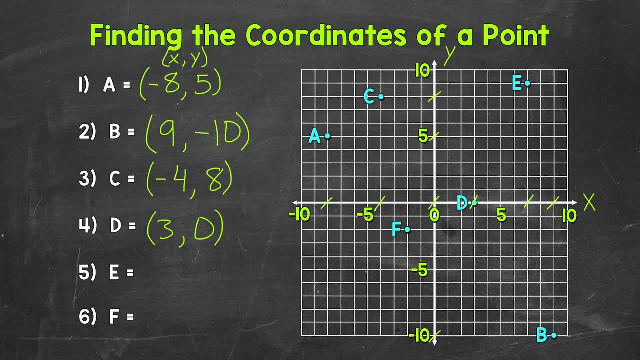 with the y-coordinate E is right here along the x-axis, So the x-coordinate is 7.. And then, as far as the y-coordinate E is right here along the y-axis, So we go over 7 and then up 9 for point E. 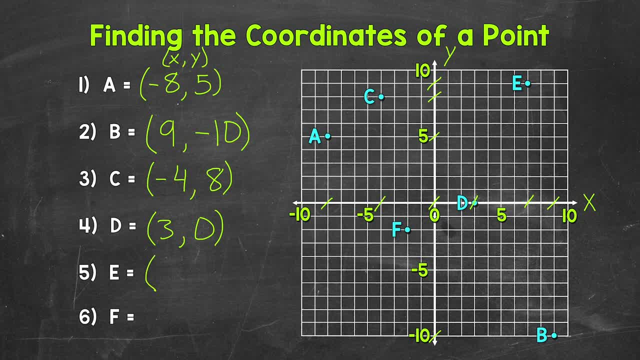 So those are the coordinates. The x-coordinate is 7, and then the y-coordinate is 9.. Lastly, let's move on to number 6, where we have point F, As far as the x-coordinate F is right here along the x-axis, which is negative 2..